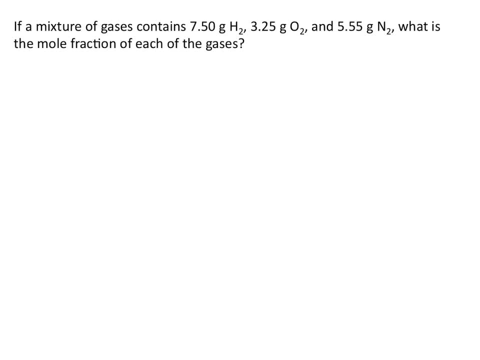 7.5 grams of hydrogen, 3.25 grams of oxygen and 5.55 grams of nitrogen. what is the mole fraction of each of these gases? If the mole fraction of each of these gases contains 7.5 grams of hydrogen and 3.55 grams? 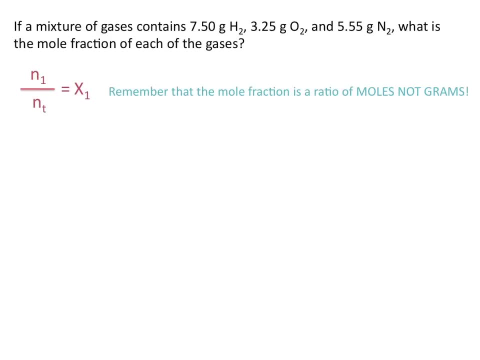 of oxygen. what is the mole fraction of each of these gases? Remember that the mole fraction is the ratio of moles, moles of one gas divided by the total number of moles of all the gases. Now, I should point out that we're calculating. 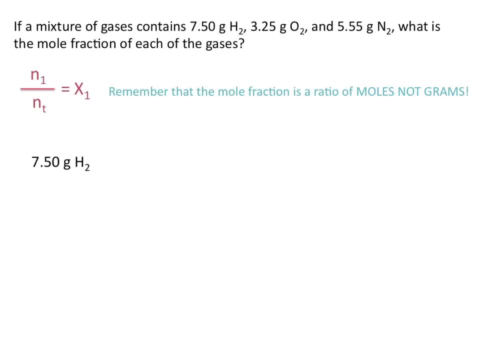 mole fractions of gases. but this mole fraction concept works for anything. You don't have to just have gases. So in order to calculate the mole fraction of each of these gases in into moles of that gas And we can go from grams to moles using the molar mass. 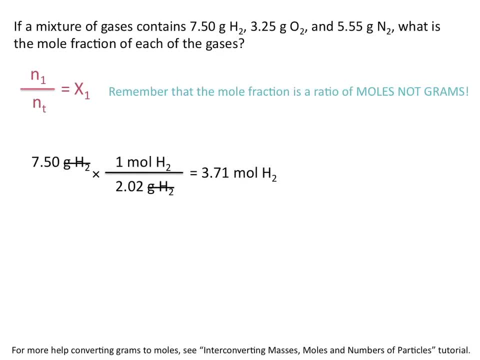 This tells us that 7.5 grams of H2 is equal to 3.71 moles of H2.. We're going to do the same for oxygen Convert to moles using the molar mass of O2.. That allows us to cancel units of grams and leaves us with units of moles: 0.102 moles of O2.. 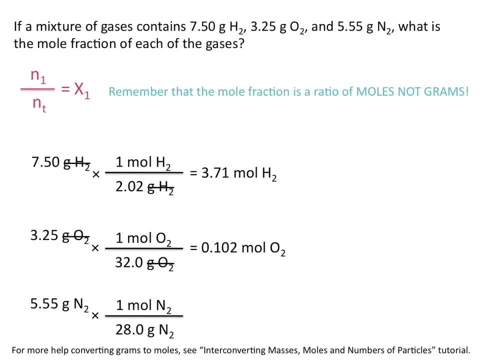 And we'll do the same thing for nitrogen, Using the molar mass of N2 and calculating that 5.55 grams of N2 are equal to 0.198 moles of N2.. Now we've calculated the moles of each of the individual gases, So to calculate the 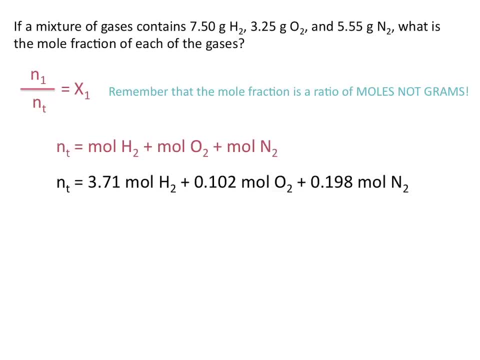 total number of moles. we're going to add these numbers together, So N sub T is equal to 4.01.. Now to calculate the mole fractions, we take the moles of each individual gas divided by the total number of moles to give us the. 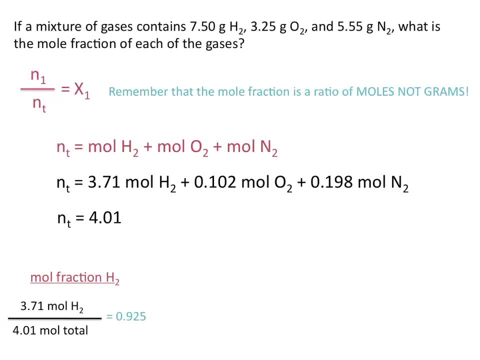 mole fractions. So the mole fraction of H2 in this mixture is 0.925.. The mole fraction of O2 is the number of moles of O2 divided by the total number of moles, which is equal to 0.0254.. And the mole fraction of N2 is equal to the moles of. 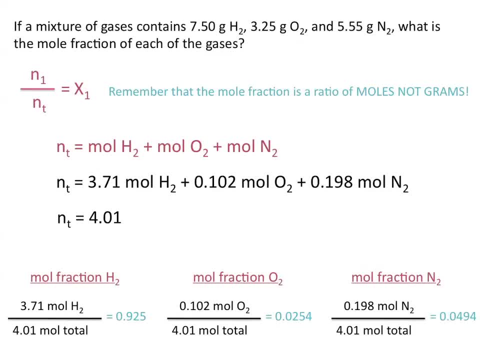 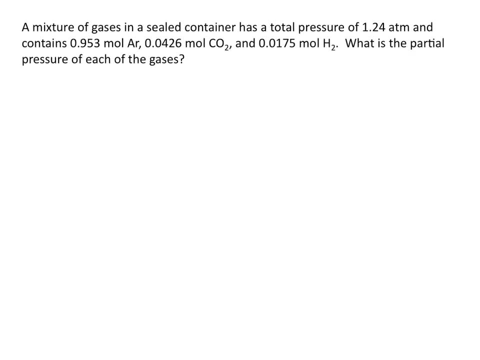 N2 divided by the total number of moles, which is equal to 0.0254.. Let's try another problem. A mixture of gases in a sealed container has a total pressure of 1.24 atmospheres and contains 0.953 moles of argon- 0.0426.